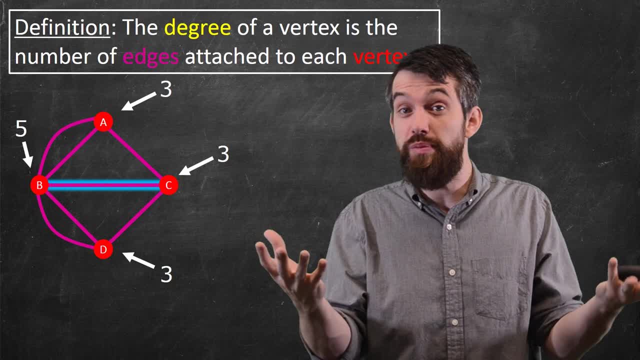 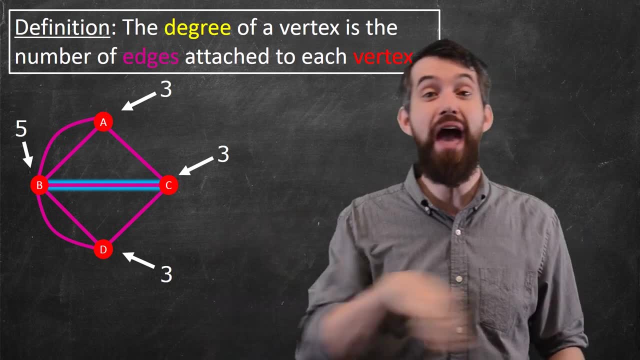 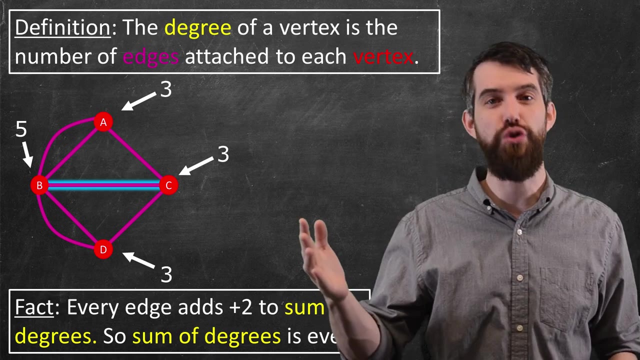 and it adds plus 1 to the degree of C because it's an edge leaving from C. That is, this one edge that we've added has actually gone plus two to the total degree of everything in the graph. So this is a key fact: Every time you add an edge, you add plus 2 to the sum of the. 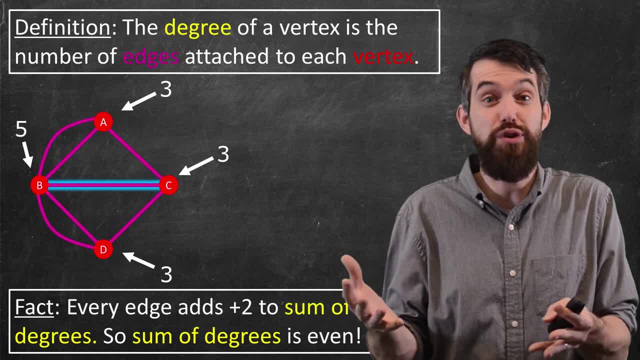 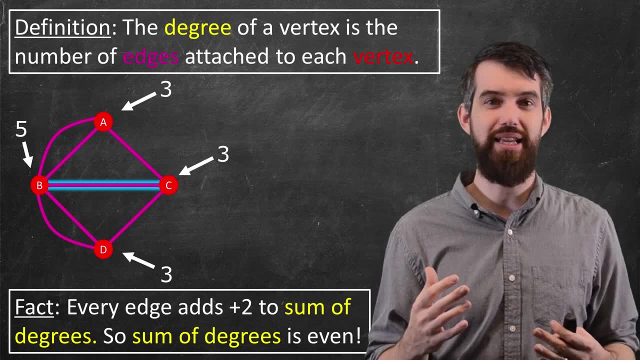 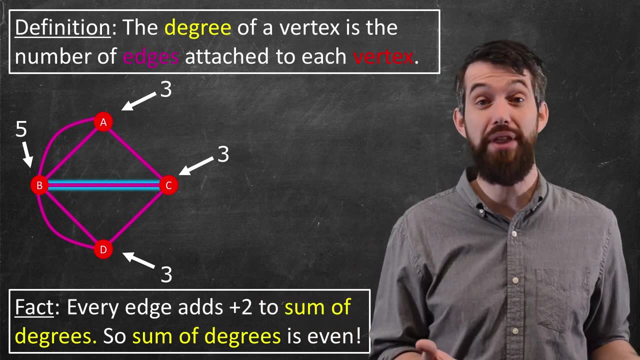 degrees of the both vertices, and so, therefore, the sum of the degrees of all the vertices has to be an even number. Now, this is going to be very important for us, because it says that a whole bunch of different graphs- the ones where the sum of the degrees would be odd- are just not possible to have as 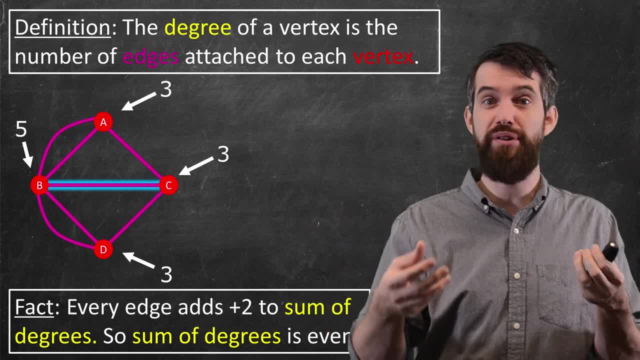 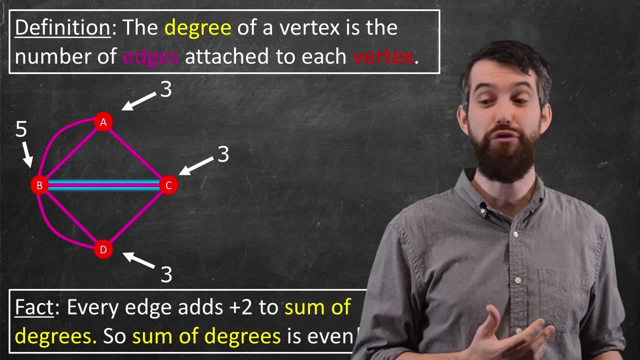 graphs, You're going to have to have some edge. that starts at a vertex and then ends nowhere, and so is not actually a graph. We can use this to rule out a whole bunch of things. So, for example, consider these two pairs of examples- I've got five people, and among those five people there's 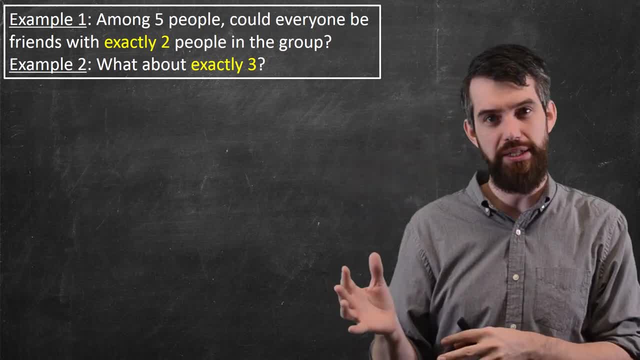 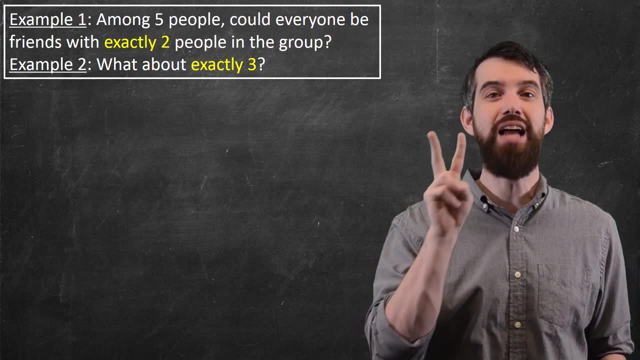 different friendships between them. Some of them are friends and some of them are not friends. And the first question I'm going to ask is: is it possible that everyone in those five people is friends with exactly two other people, Not three, not one, exactly two. Okay, so let me begin. 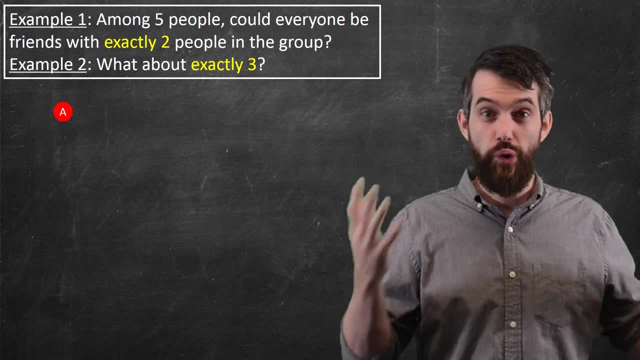 with some person called A. Now this person. the rule is that they have to be friends with two other different people, So I'll put two other people here. So I'll put two other people here. So I'll put two other people here. So I'll put two. 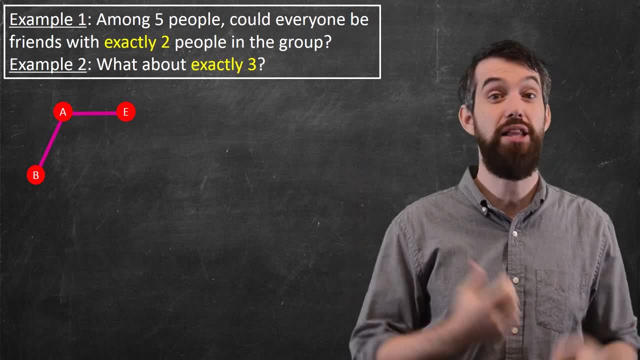 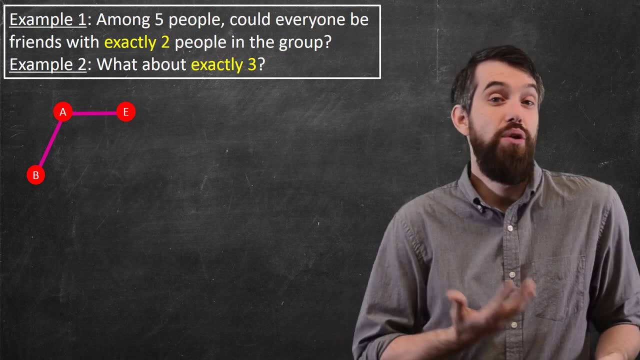 people that they're friends with. I'll call them B and E. And now let's think about B. Well, B is already friends with A. wants to be friends with one other person, so why don't I go and say that they're friends with someone called C? C's friends with B and maybe one other. how about D? And then? 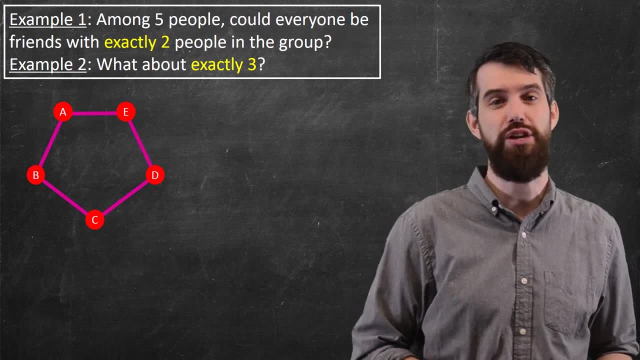 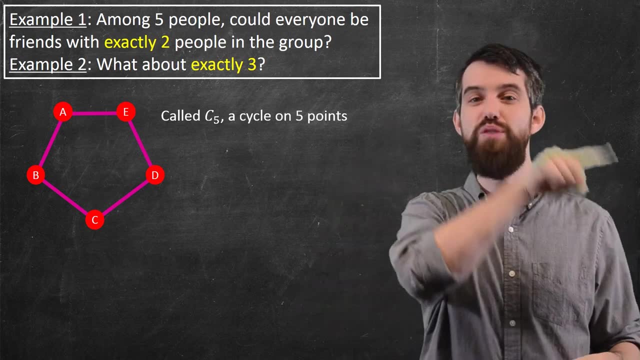 D's friends with C? how about one other? Well, E is the natural choice. This, by the way, is called a cycle, the cycle C5. It's one where you've got sort of a arrange them all in a circle and they're. 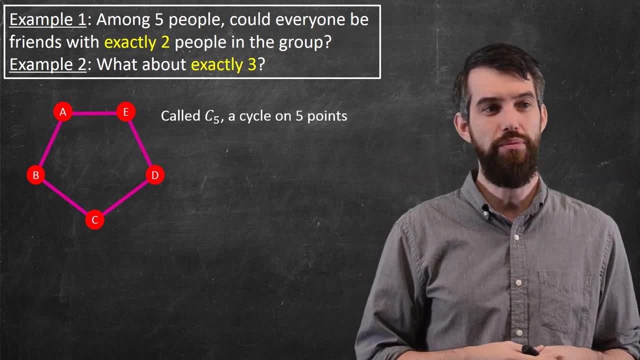 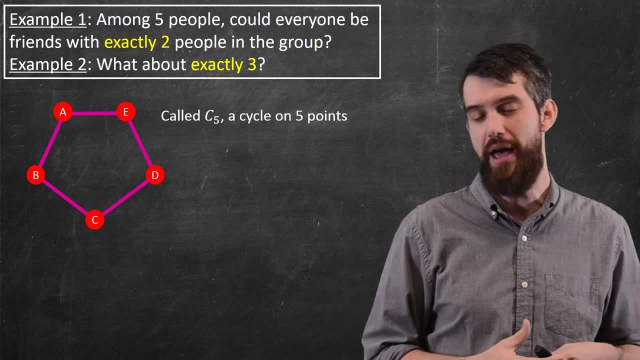 all connected exactly once. That's what a cycle is. So we didn't necessarily come up with the only answer to this. We might have to investigate whether some other ones are possible. You could pause and try that, But this is one answer at least to whether it's possible to make such a.